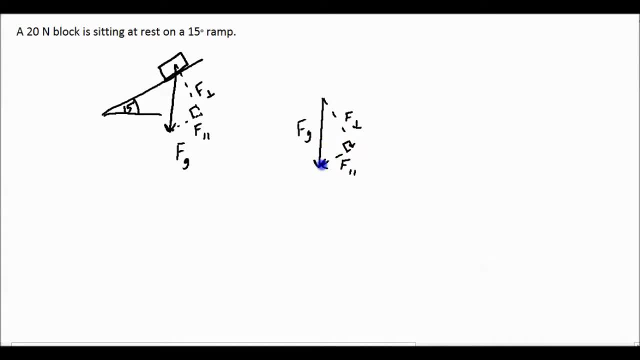 So this one's going down and this one's going also down because it's gravity, They all go down. Now the question we have to establish is: what is this angle right here? Because what's going to happen is this parallel force is going to be a right angle. 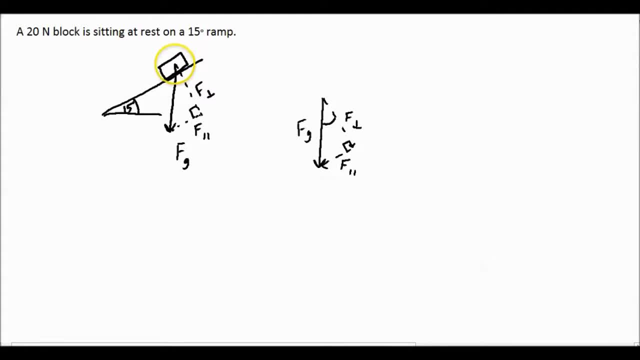 This parallel force is going to be equal to this parallel force right here. That is the direction of the parallel force of gravity, That is the one that is pulling the block down the ramp. If the block is at equilibrium, then we can easily right now say that the force of friction is equal to that. 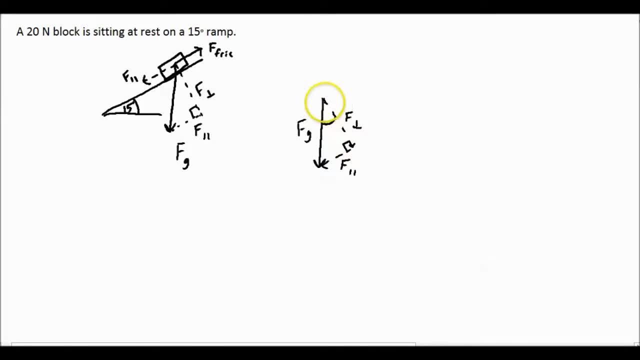 And if it's at equilibrium, then this side of the triangle right here indicates the perpendicular force of gravity and we can say that our normal force is that long. So we have our diagram drawn, but we don't know any numbers yet. So the question is: what is this angle right here at the top? 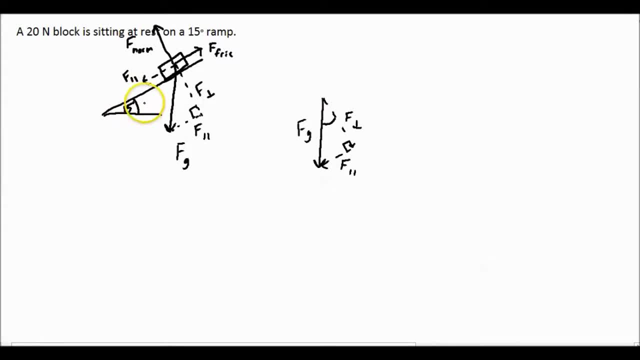 And the thing to keep in mind is that this 15 degree angle of the ramp basically translates to this angle right here, because 15 degrees is how much the ramp is off the ground. So the ramp is off the ground, And so 15 degrees is how much the downward force of gravity has been changed. 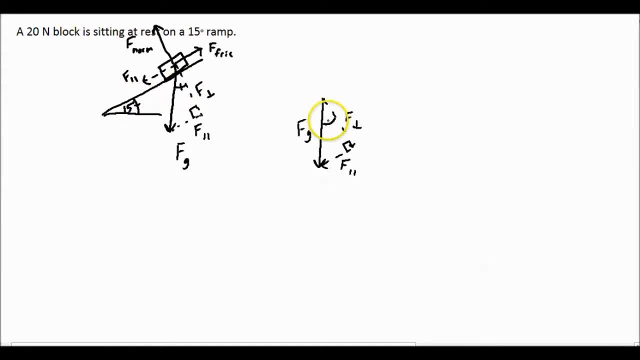 So this right here is the same exact angle as that, And this is all 15 degrees. So this is our theta right here. So theta is 15 degrees, Our Fg, which is equal to our hypotenuse, because it's opposite of the right angle. 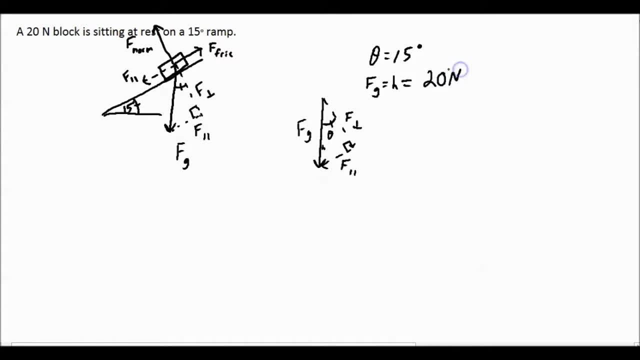 is equal to 20 Newtons. Our F perpendicular is our adjacent side And our F parallel is our opposite side. So we can fall back on our old equations: h times the sine of theta is equal to our opposite side And h times the cosine of theta.